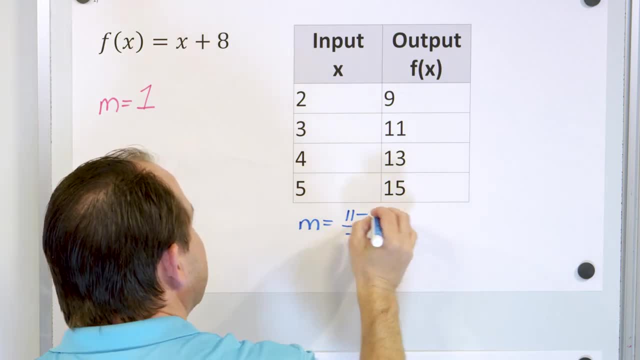 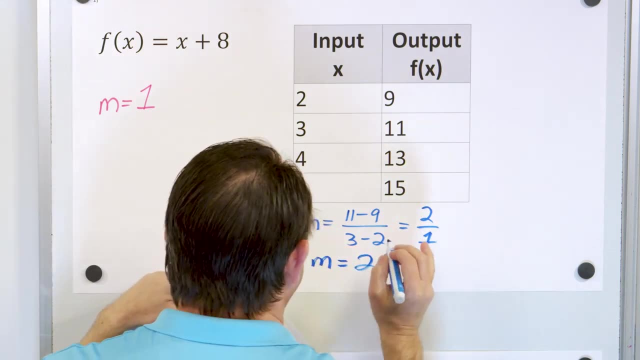 so 3 minus 2.. And 11 minus 9 is 2., And on the bottom we get a 1., And so the slope here is 2.. All right, So if we have one function with a slope of 1 and a 1, another. 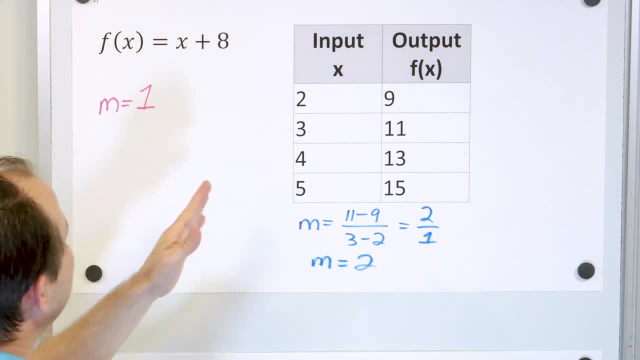 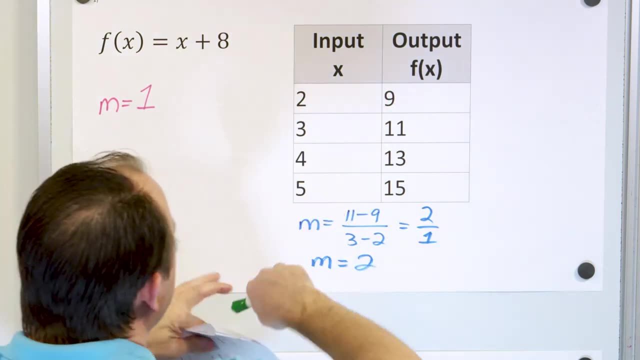 totally separate function with a slope of 2, then which one has the higher rate of change? It would be this one, the one that has the larger slope. So instead of writing down a bunch of words, I'm just going to circle this one and say, OK, this one has the greatest or the higher rate of. 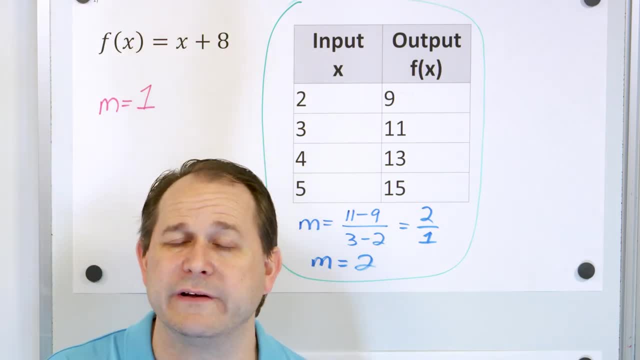 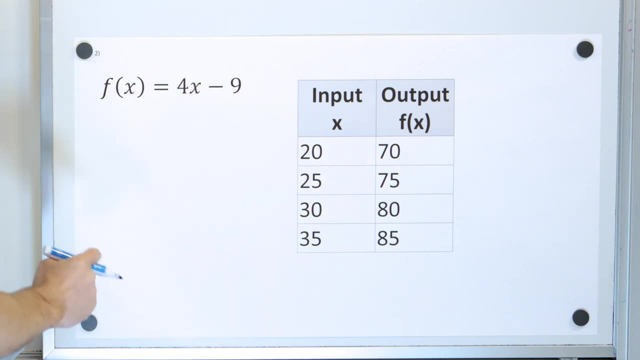 change In every one of these problems, whichever one I circle is going to be the one with the greatest slope or the highest rate of change. All right. Problem number two: we have a function here, mx plus b form, and we have another function in a table. 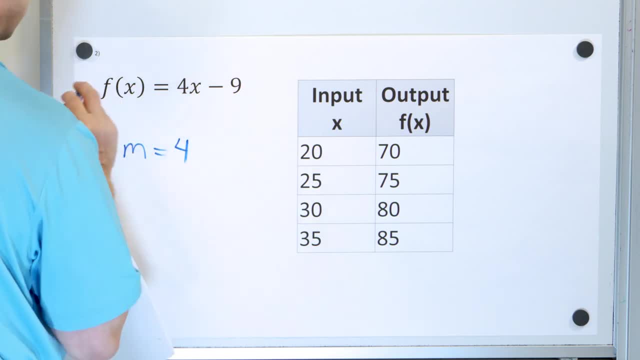 So this guy right here, it's mx plus b. The slope in this case is 4.. What's the slope down here? We have to calculate the slope And we can use any two points in the table we wish. I'm going to. 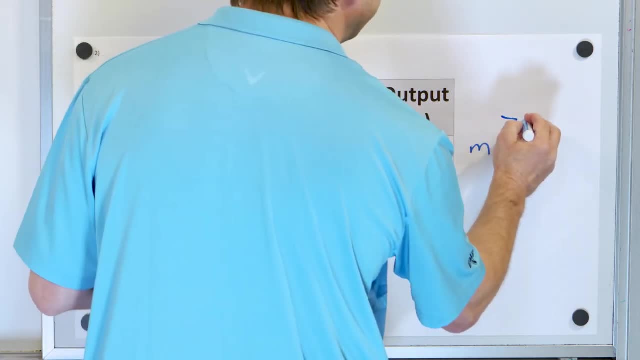 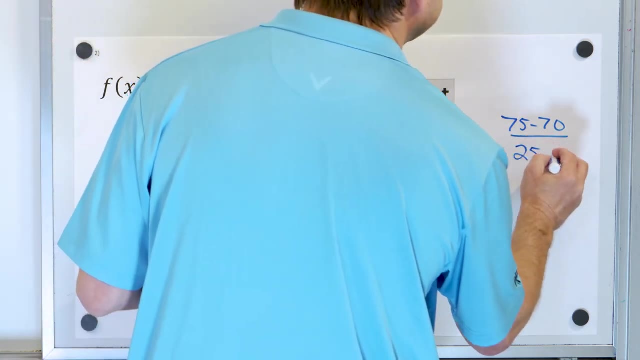 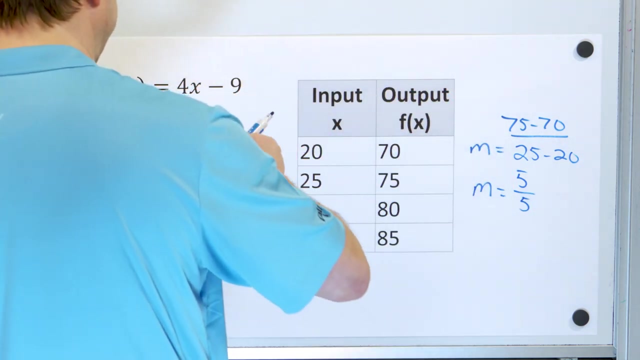 choose these smaller two numbers, so 75 minus 70. We subtract the output or the y values and then, going the same direction, 25 minus 20.. And so what we get here is a 5 on the top and a 5 on the bottom, And so let me just double check myself before I go any farther. 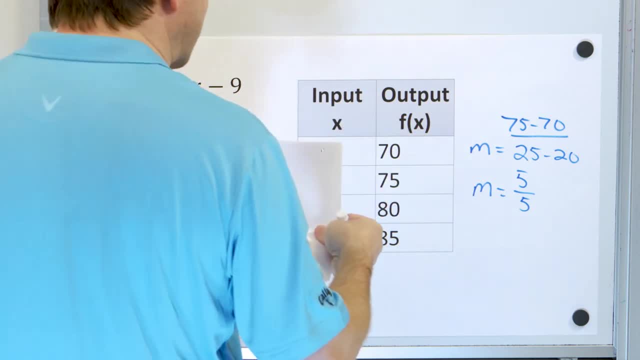 because you know, I make mistakes all the time, So I just want to make sure that there's no problems. The slope that we get right here is indeed 1. That's correct. So which one has that larger or the highest rate of change? 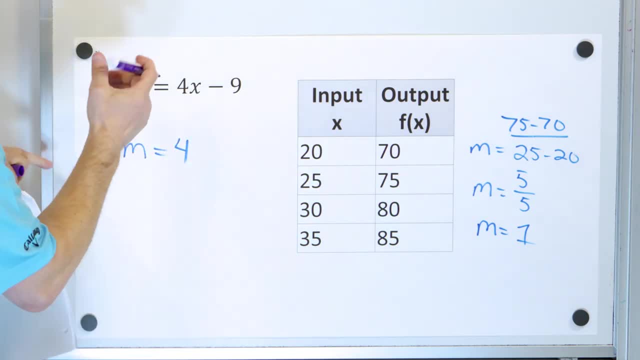 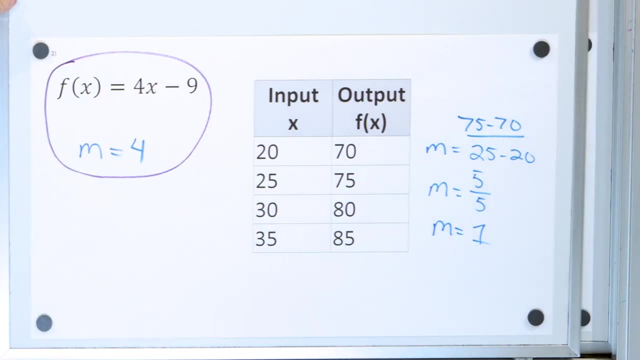 The slope of this is 1, and the slope of this is 4.. This one has the higher rate of change. We're always going to be circling the function that has the higher rate of change, and that is it All right. Let's take a look at problem number. 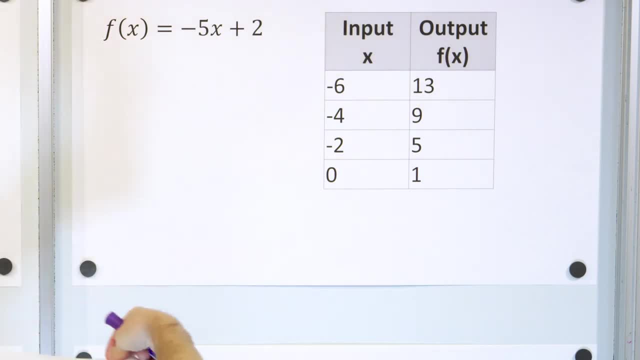 three. So what is the slope of the equation here? mx plus b. Basically, the slope here is in this case negative 5 right here, Which means this guy slants in the down direction. And what is the slope over here? So I'm going to 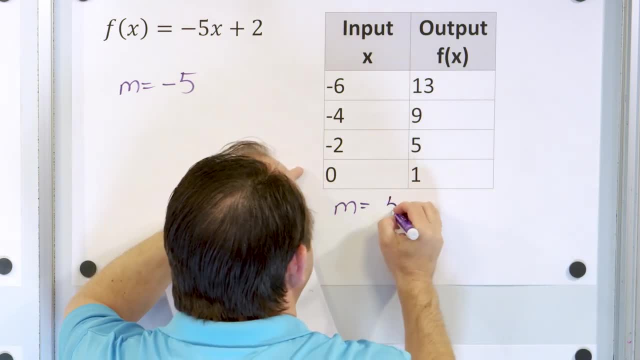 choose these numbers down here. I'm going to go 5 minus 1.. That's the output: 5 minus 1.. I have to go the same direction: negative, 2 minus 0.. 5 minus 1 is 4, and then negative. 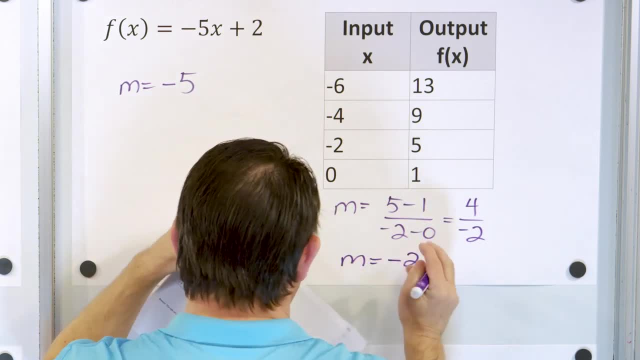 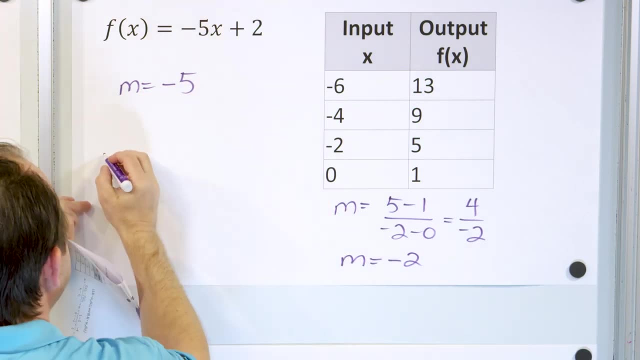 2 minus 0 is negative 2.. So the slope is actually negative 2.. So which one's bigger: negative 5 or negative 2?? I know you might be tempted to say this one because there's a bigger number, But if you remember your number line, if this is 0,. 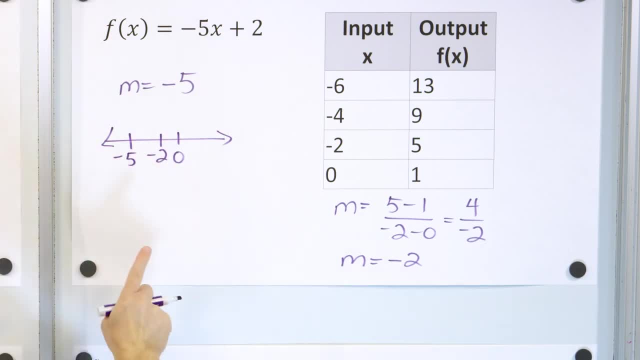 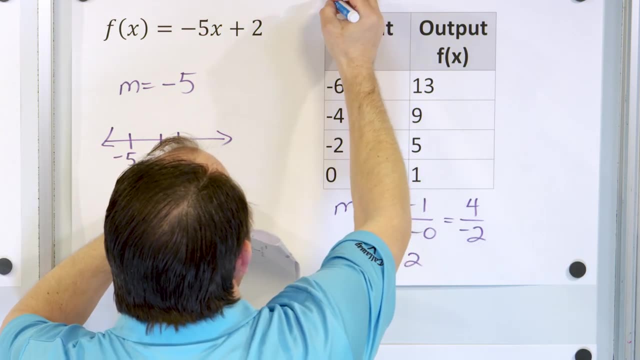 then over here is negative 2, and somewhere way over here is negative 5.. Which one's bigger? Actually, negative 2 is bigger, Negative 2 is bigger, so that has the larger rate of change. So in this case this one is the highest rate. 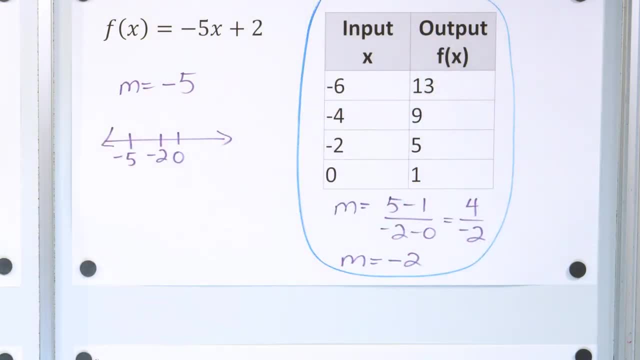 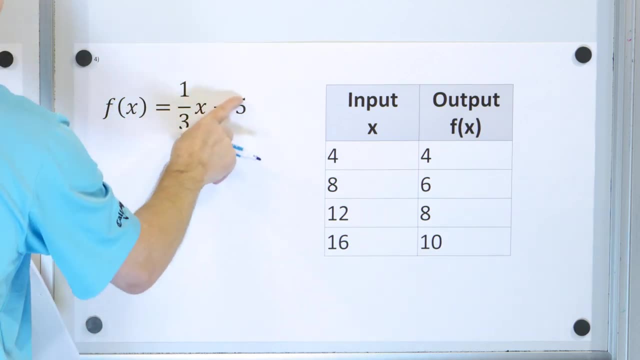 of change of these two functions, the one in the table. So that's the final answer there And, believe it or not, this is our very last problem. What is the rate of change of this function? mx plus b? The rate of change of the slope is 1 third. 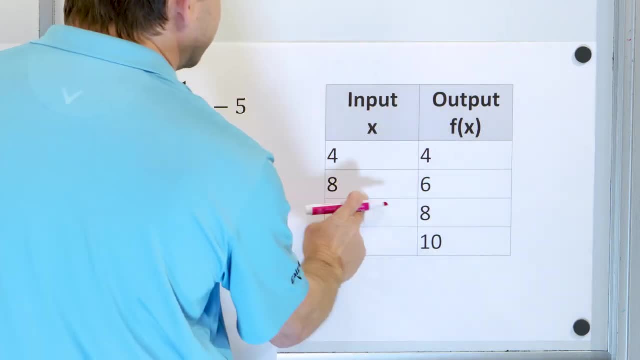 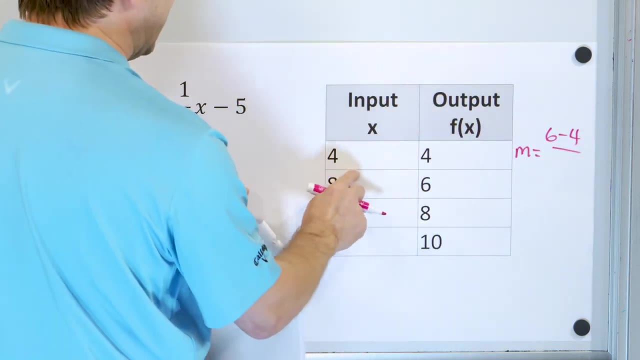 And then we have to calculate the slope over here. I'm going to use these numbers here. The slope is going to be 6 minus 4 on the top and then, going the same direction, 8 minus 4 on the bottom. 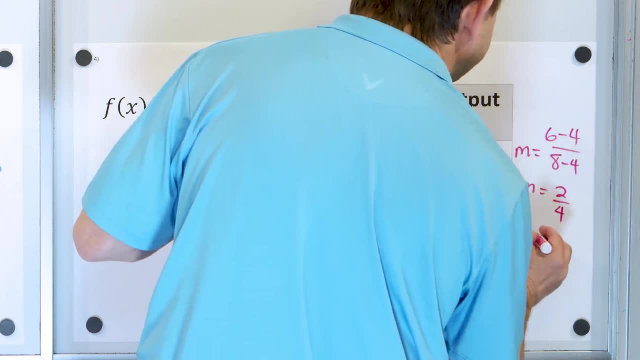 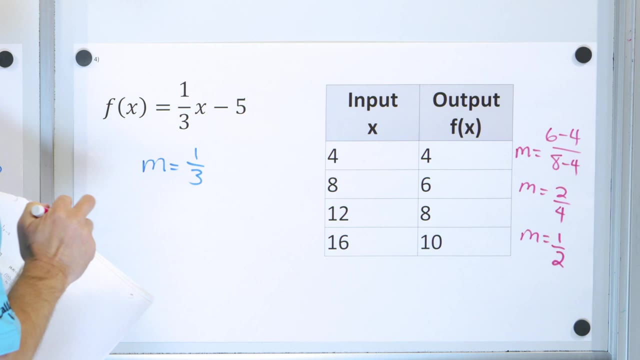 So the slope: on the top you get 2.. On the bottom, you get 4.. And you simplify this fraction to 1 half. So which one is bigger, 1 half or 1 third? The number 1 half is bigger. 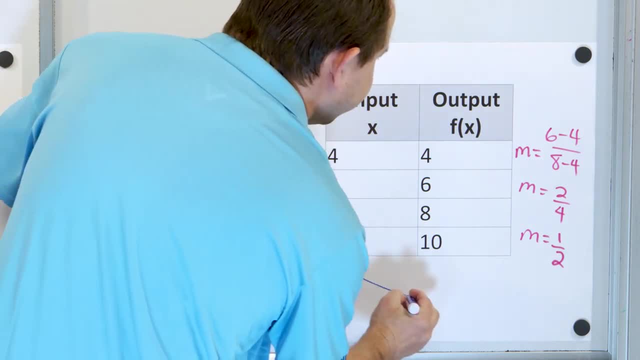 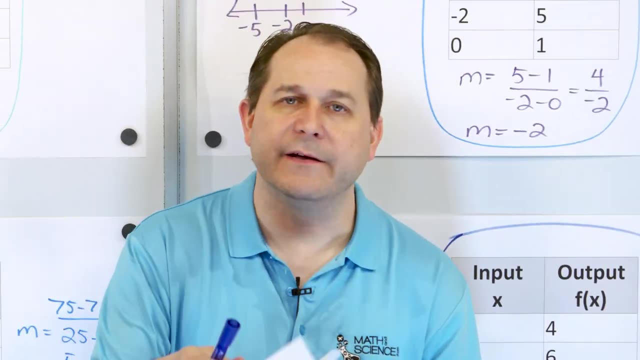 It's bigger than 1 third. So actually this is the larger rate of change of these two functions here. So you might say: why are we doing this lesson? It's because we've already done this before. We know how to find the slope of an equation in slope intercept. 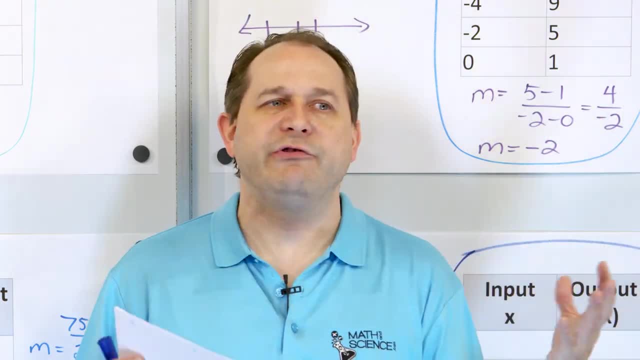 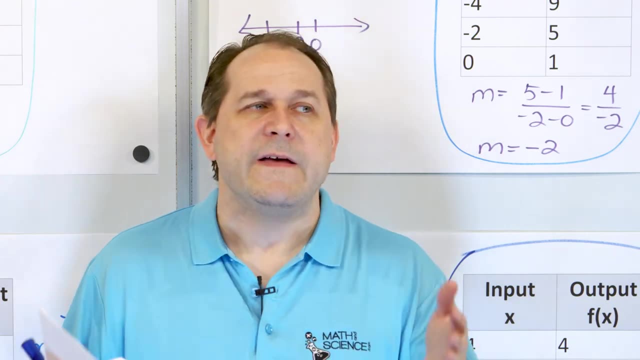 form. We know how to find the slope from numbers in a table. We're just doing a different type of problem to give you practice with it, but also it's the kind of thing you might see on a standardized test or an exam as well. 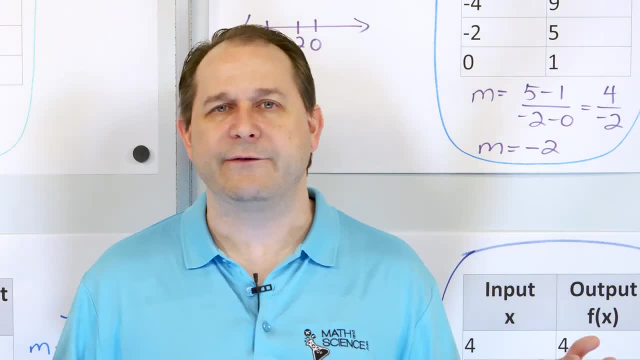 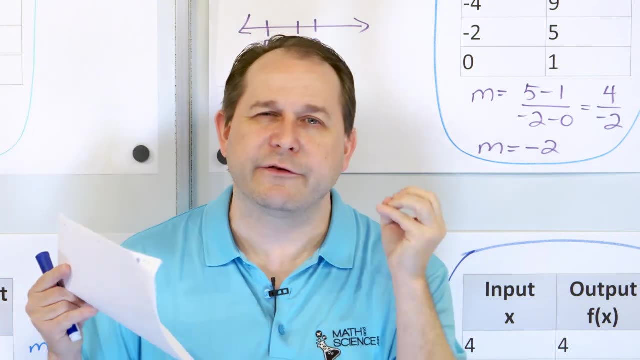 Give me two different lines in different forms and tell me which one has the greatest rate of change, or the greatest slope, or the smallest slope or whatever it is. So we're practicing pulling that info out and also comparing them And we understand that whatever answer, we circle actually. 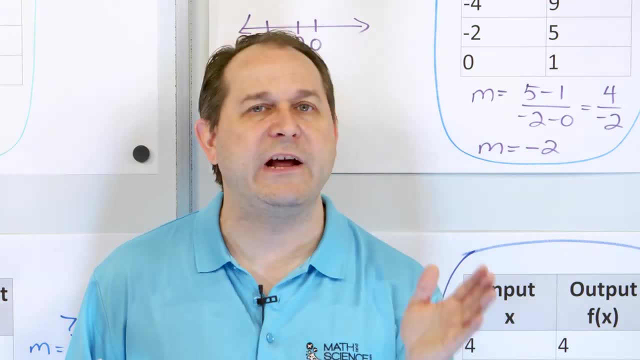 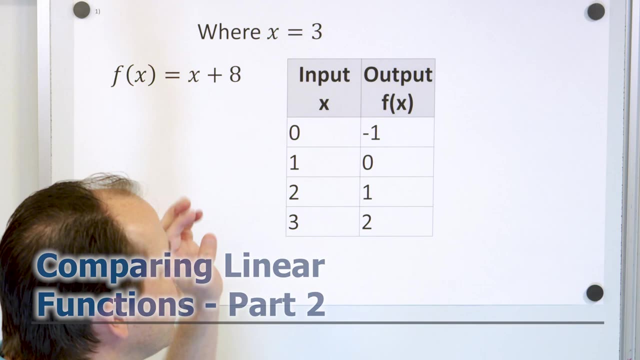 has a steeper graph if we were to graph them, because higher rate of change, higher slope, means steeper graph. So solve these. Follow me on to the next lesson. We'll continue to build your skills, And here we're not going to be comparing their rate of changes. 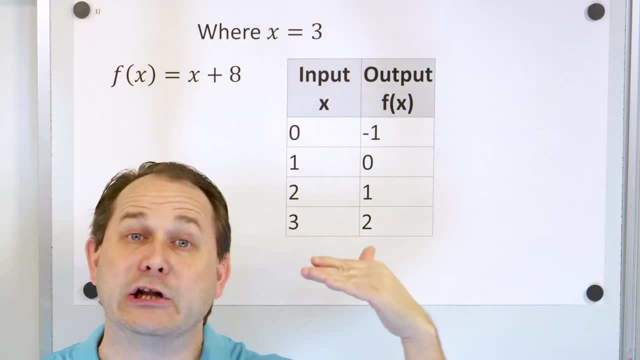 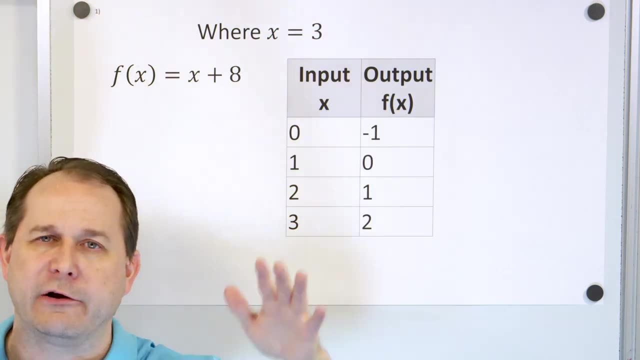 or their slopes. We're going to be comparing which of these two functions has a larger value when x is greater than 1 half. We're only trying to find out the difference, and that's where we do a test as well, And we usually try to find out the difference. 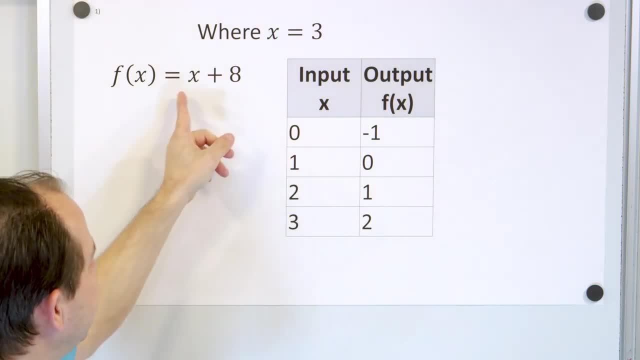 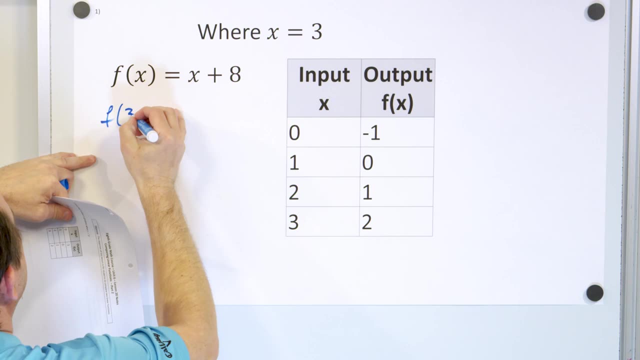 based on what is going on: benefit by function, return upon return. Now, in other words, what we want to do with our Sol opportunities is we want to identify a point of value that's a depth less than 2 of that 3.. 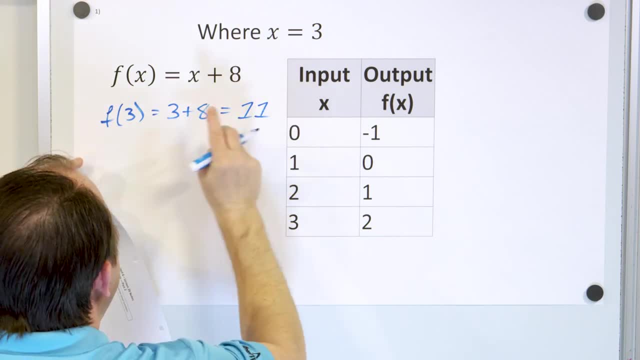 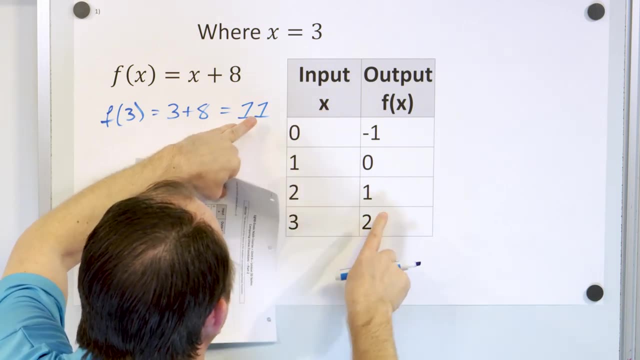 And we want to размер that to at least an больш. so it doesn't take us to the point where we want to Jon and D Owen to experiment. So what do we do with it? Because we're all meant to And we're not going to do it. 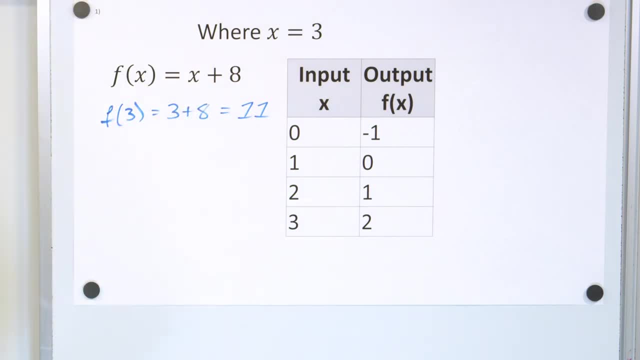 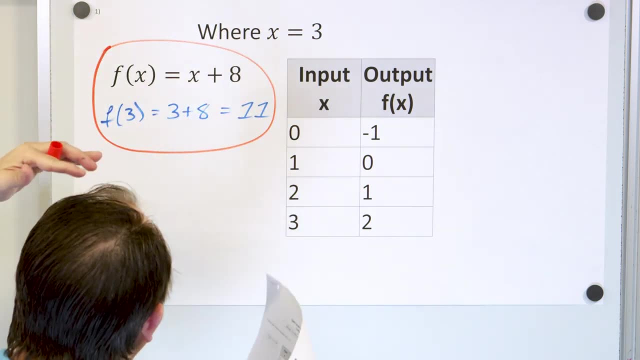 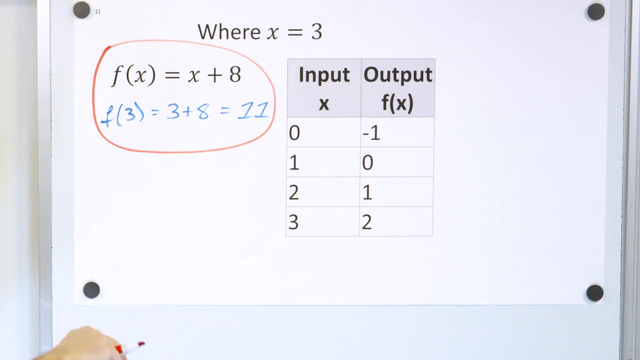 is bigger? of course it's this one, because that's all we care about here is which of the functions is larger, which one has a larger value, not the rate of change, not the slope, the actual. the actual value of the function when X is 3 here is 11. the value of this function when X is 3 is only 2. so that is the. 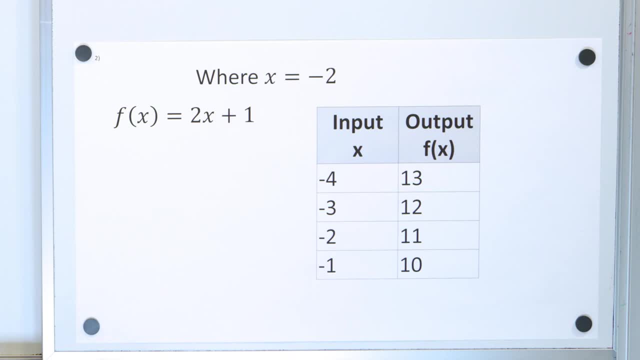 final answer. all right, let's take a look at problem number 2. here we have a function and we have a table which is a different function. let's compare these functions: when the input is allowed to equal negative 2, which one has the greatest value at that moment. so we can evaluate, when X is equal to negative 2. 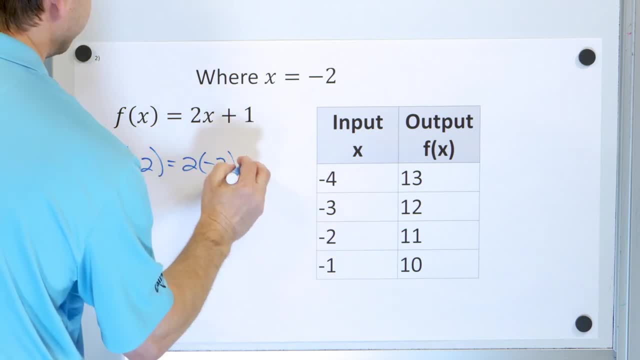 we'll say 2 times negative. 2 for X means we'll have negative 4 here plus 1, and then we have negative 4 plus 1 is negative 3, so the output there is negative 3. but when X is equal to negative 2 in this table, the output is: 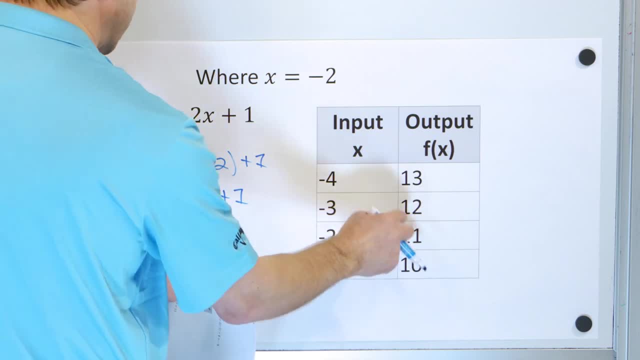 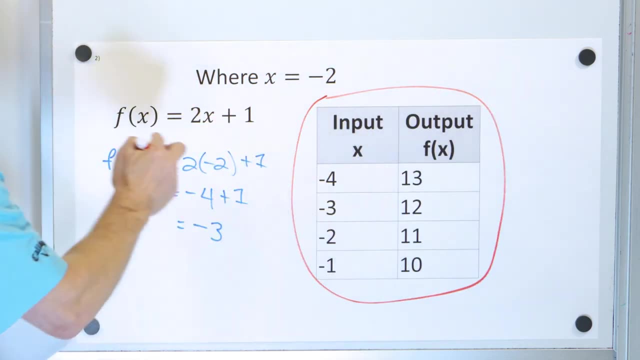 11. so which of these two has a larger value? this one does over here you. so actually this function has a larger value when the input X is allowed to be negative. 2. all right, let's take a look at problem number 3. we have a function. 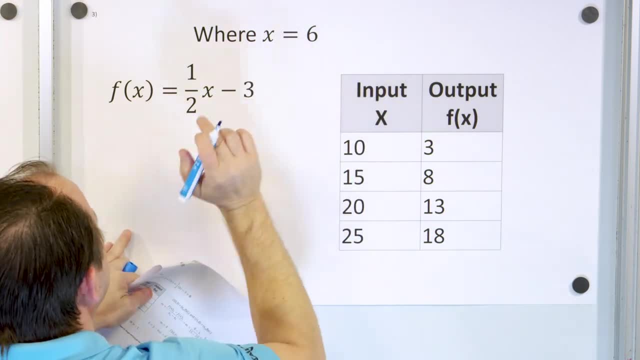 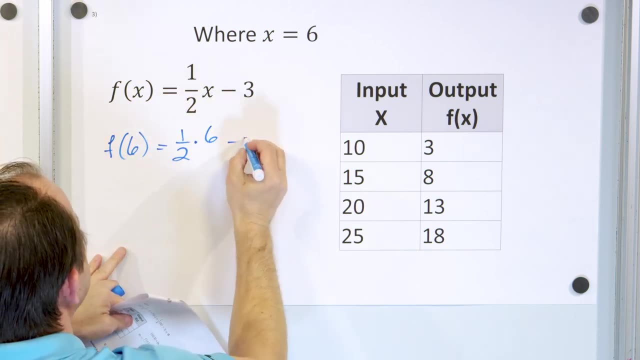 here and a function in the table: which one is larger when X the value is allowed to be equal to 6. well, first we have to calculate when X is equal to 6 here. well, we have 1 half times 6 minus 3. 1 half of 6 is 3 and we have minus 3 and 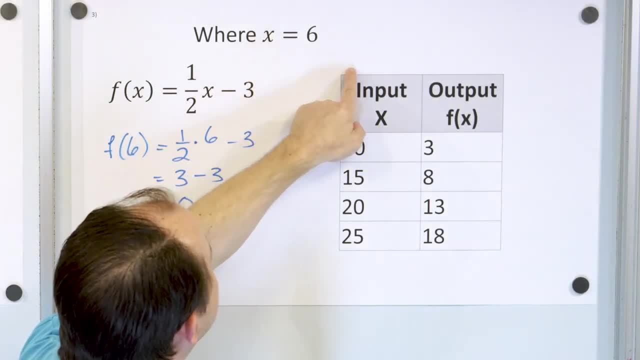 so the output here is actually 0. so the next step would be to figure out in this table what is the value of this function when X is equal to negative 2. so this is negative 3 and we're left with negative 2, we're left with negative 3, we're left with negative 3. 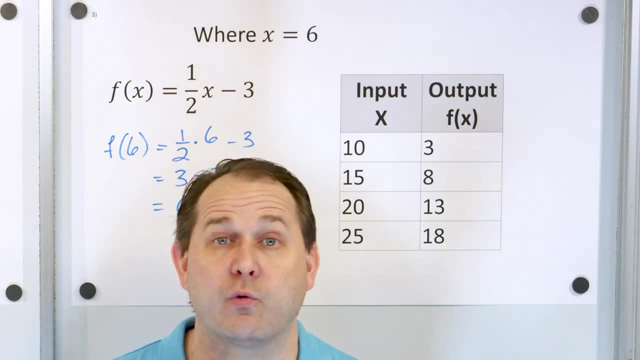 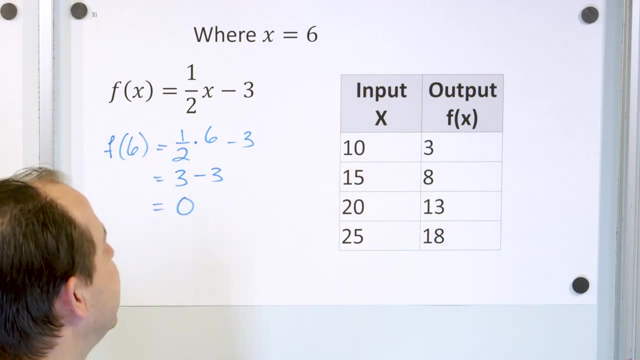 we're left with positive 2, are we right? we're right. we're left with negative 3. by all. that means we have this function here. what's the value of this function? if we look here, we have the value of this function. we have a random. 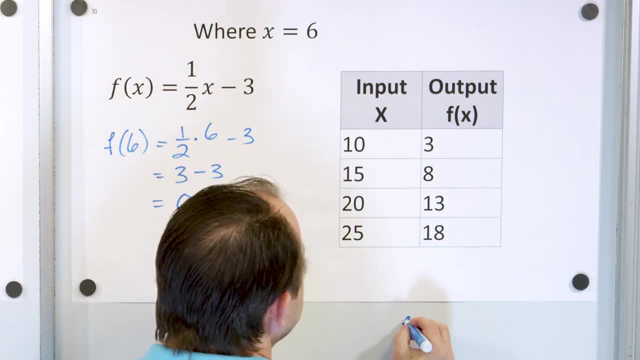 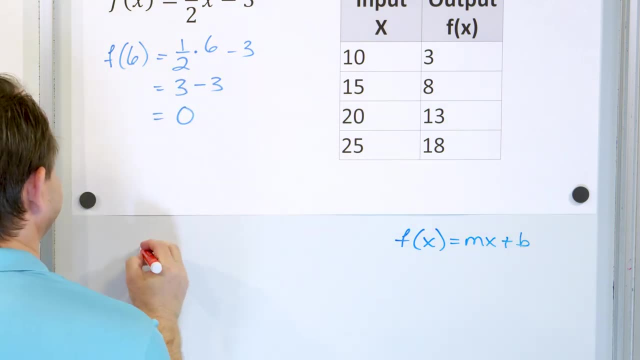 value in this function. so we can find the value of this function. what happens when the input is allowed to be 6? but I don't have a value when the input is 6, so your first thought would be: well, there's a mistake, the table is wrong. 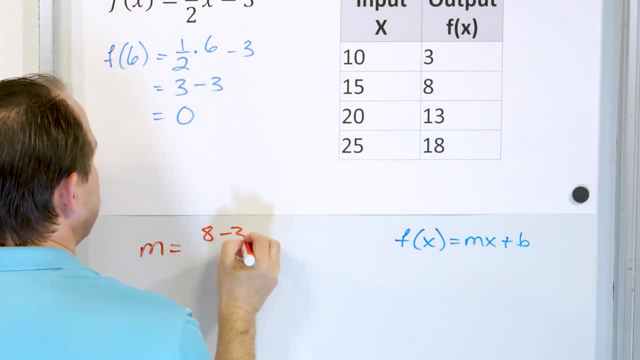 it's not. it's not complete, but remember, when we have enough information to write 3 and the bottom two points 15 minus 10. so we get a 5 on the top and a 5 on the bottom, so the slope is equal to 1. so then we can take that slope and put it. 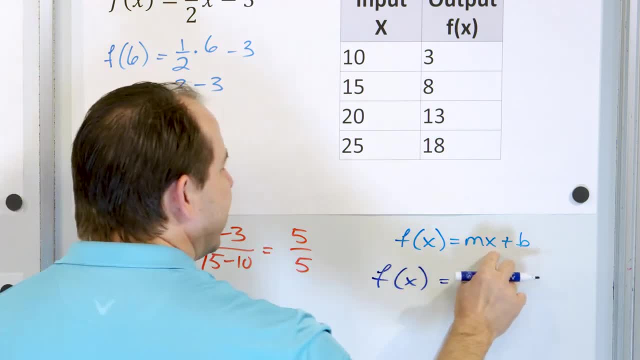 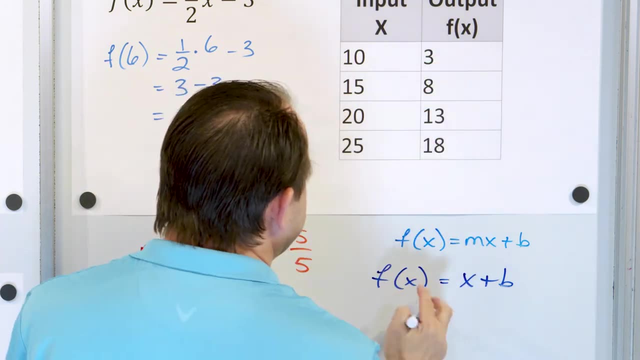 in here and say that the slope is 1 times X. so we have X plus B. now to figure out what the function is, we have to pick a point and put it in here. the output is 3 when the input is 10. we've done these kinds of things before. let's. 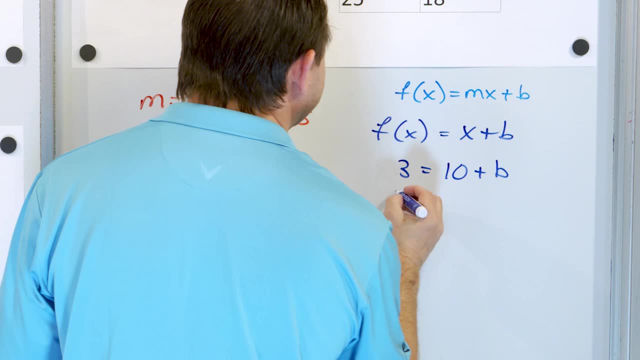 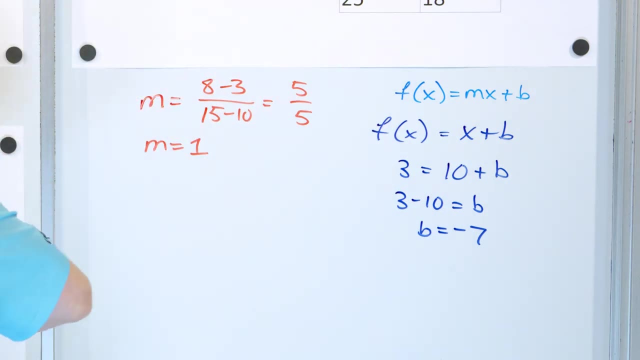 solve for the y-intercept. all right, we're gonna subtract 10, so 3 minus 10 is equal to B, so B is equal to negative 7. now all of that work was just to help us figure out what that function actually is. in X plus B, the slope is 1 times X. 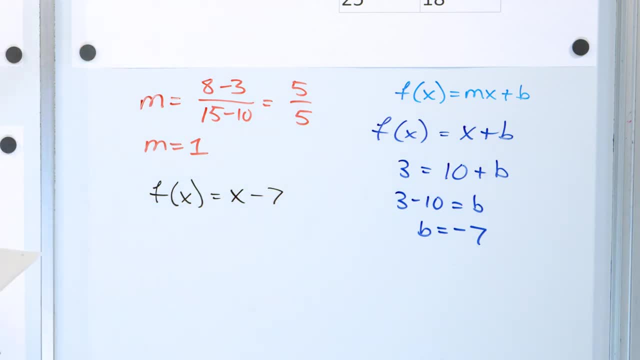 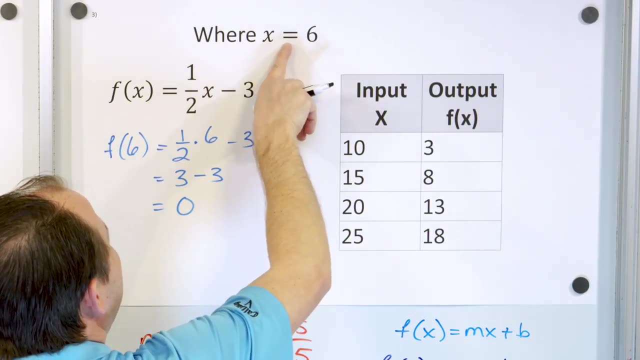 plus B, which is negative 7. so the value we get for the function is X minus 7. and then what happens? we're trying to figure out what the value of that function is when X is equal to 6. so let's put the value of 6. 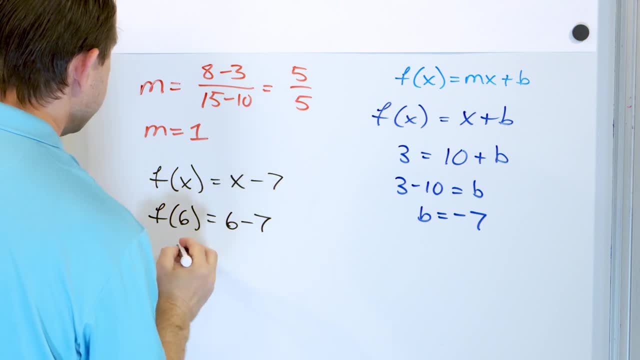 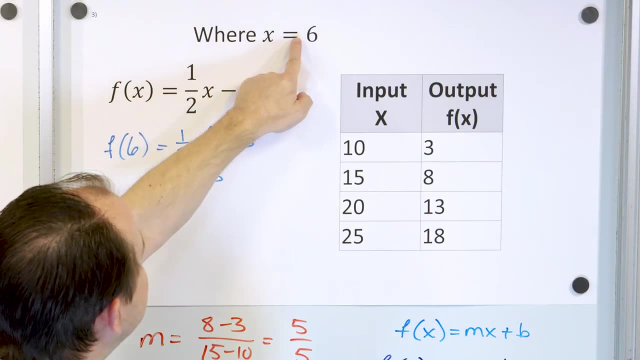 in here, you get 6 minus 7, and so the output there is negative 1. the output you get is negative 1. so what we have figured out is that when we put a value of 6 for X into this function, we get 0. when we write down the line that goes: 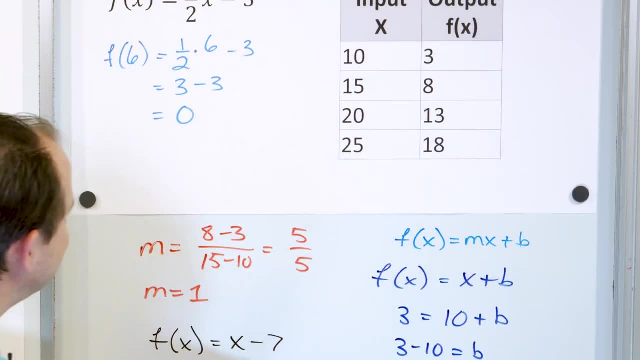 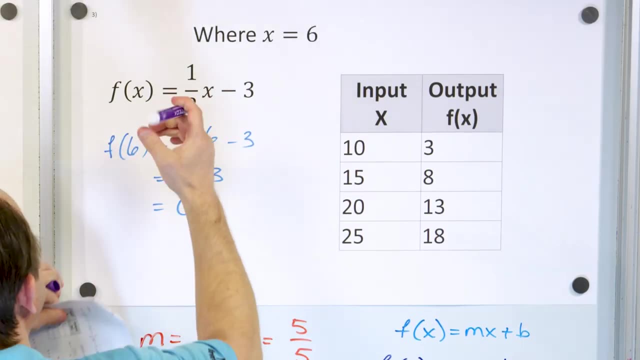 through these points and then stick a value of 6 into the input. what we get is an output of negative 1. so which one is bigger, 0 or negative 1? of course 0 is actually bigger, so this function is the larger function when X is equal to 6. all right, kind of a long-winded kind of thing we have to do. 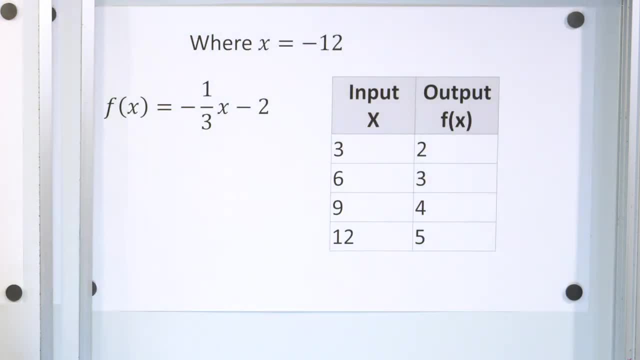 but that's what we had to do. all right, we're gonna have a similar situation here. let's take a look: when X is equal to negative, 12 means I have negative 1, 1, 3rd. then I'm multiplying by negative 12, and so negative times: negative is positive. 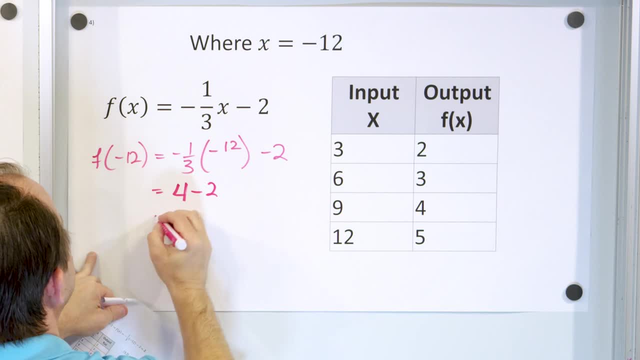 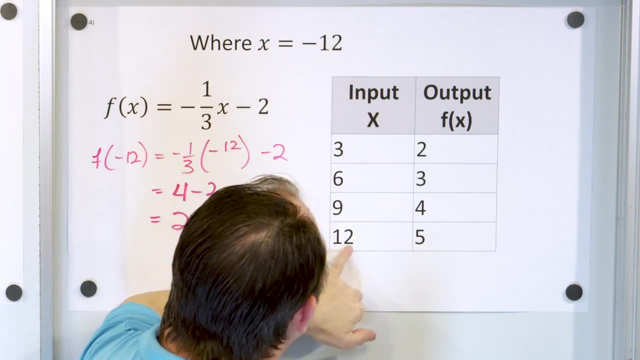 12 divided by 3 is 4 minus 2, so the output I get right there- is actually 2. Now I would like to figure out, when x is equal to negative 12, what the output is. but I don't have a value of negative 12 here. 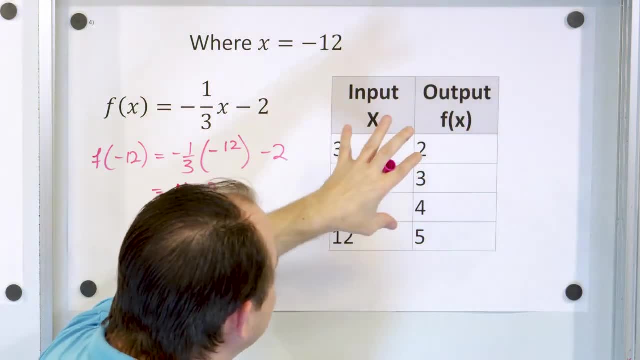 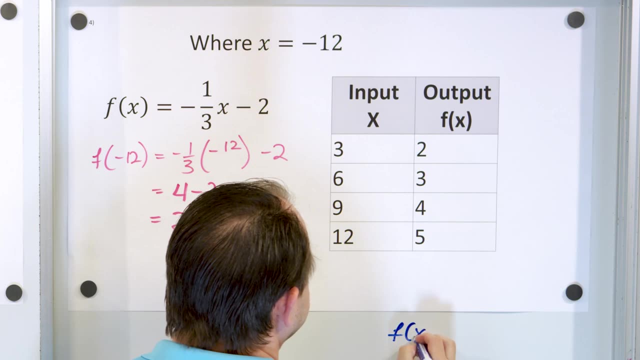 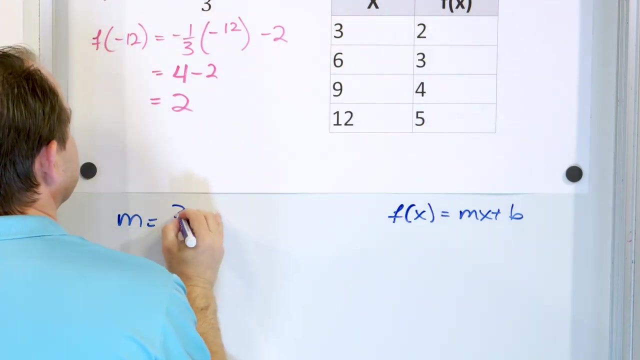 I just have additional data points. So we need to find the equation of a line that goes through these points and then stick in the input when x is equal to negative 12.. So we know that it's mx plus b. We know we can find the slope 3 minus 2 on the output and 6 minus 3 on the input. 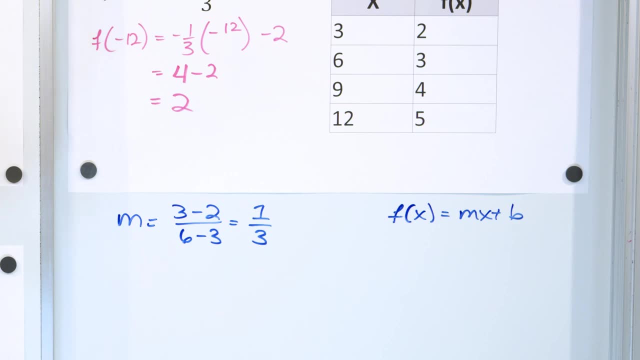 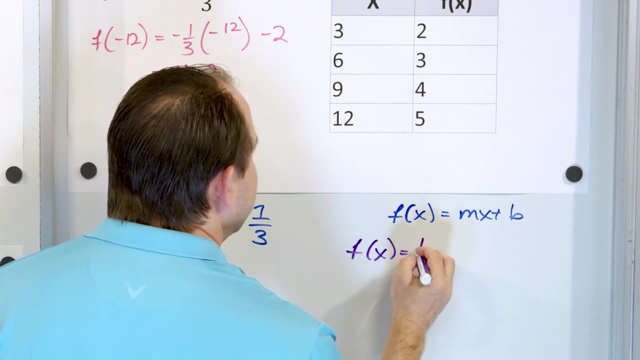 We get a 1 on the top and a 3 on the bottom, So the slope is actually 1 third. Now what we do is we stick that slope in here and we say that the function is m, which is 1 third x plus b. 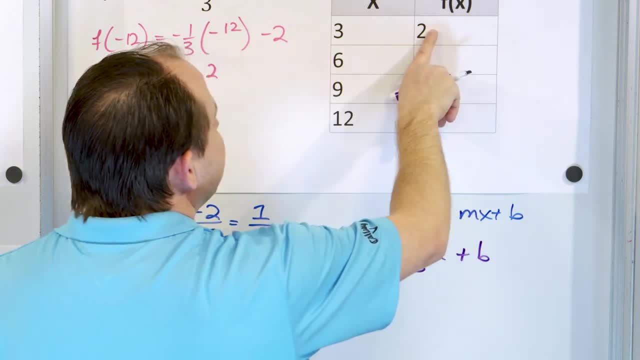 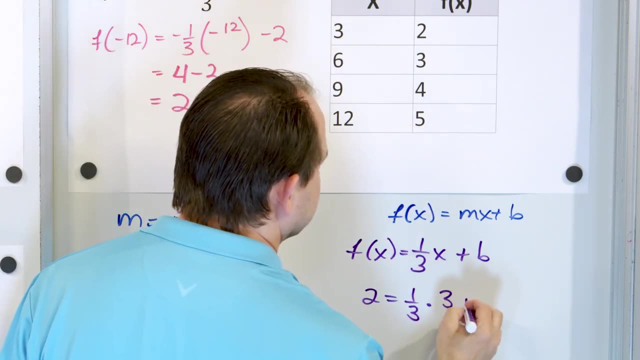 And then we can use any point we wish. we're going to use the first one here to find b. So the output is 2 when the input x is 3.. And so what we get- 1 third times 3- is just 3.. 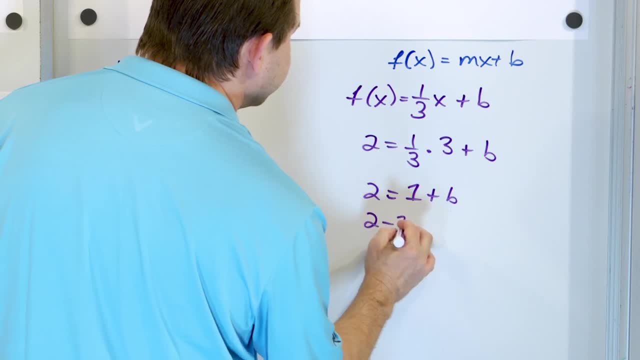 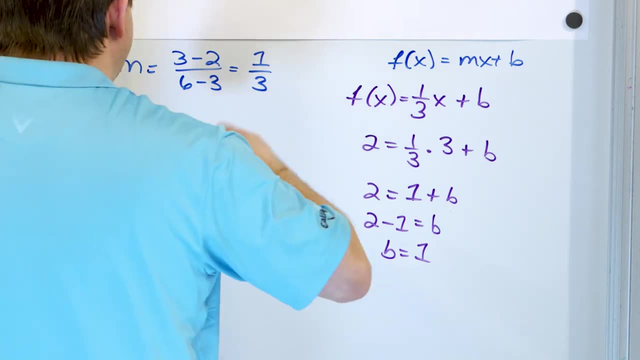 So it's 1.. And how do we find b? We subtract 1 from both sides, So b is equal to 1.. The y intercept is equal to 1.. Now why do we do all this stuff? Because now we can write down that second function, mx plus b. 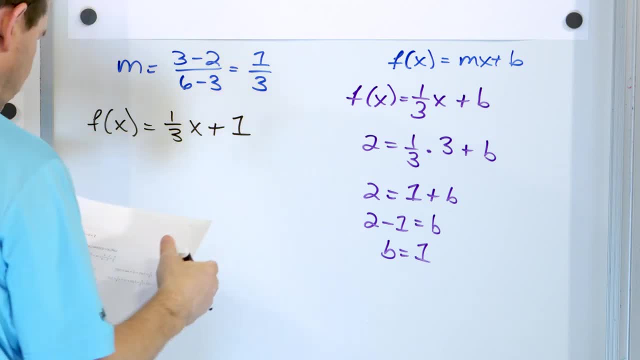 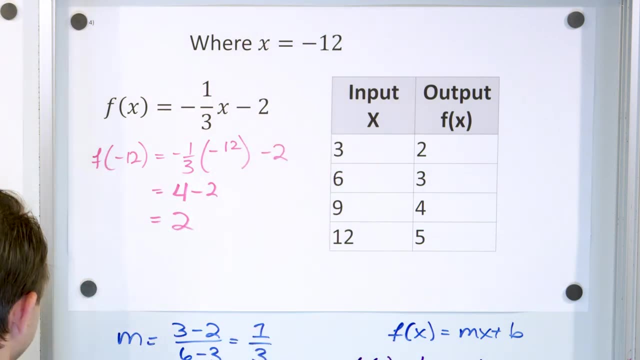 The slope is 1 third times x plus b, which is 1.. Now what do we do with that information? We want to figure out what the value of this function when the input's negative 12.. So we put a negative 12 on the input. 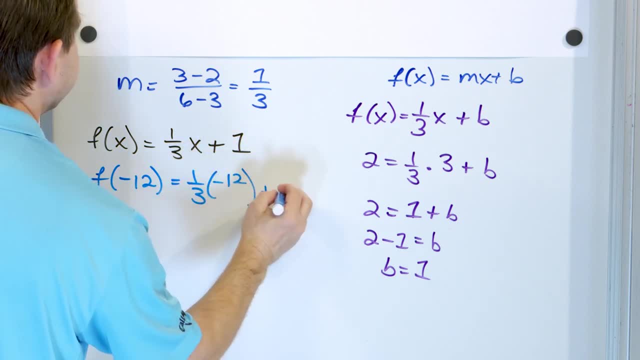 One third Times negative 12.. What do we get? 12 divided by 3 is 4, but we have this negative, so it's going to be negative 4 plus 1.. And what do we get? We get negative 3 on the output.